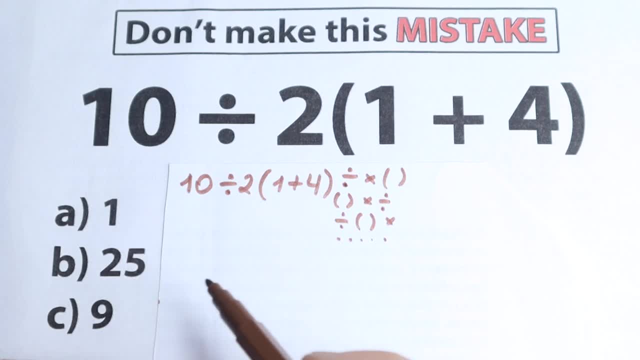 so the same answers, the same options, but different answers. so we cannot say like that In math we need to know what we how can we solve this correctly and according to a correct order of operation, because a lot of combinations right here and we need to solve it according to a correct. 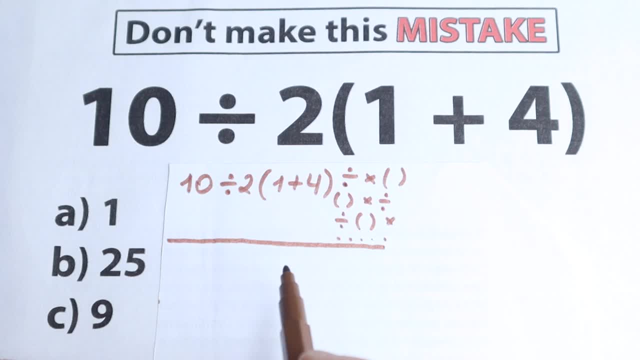 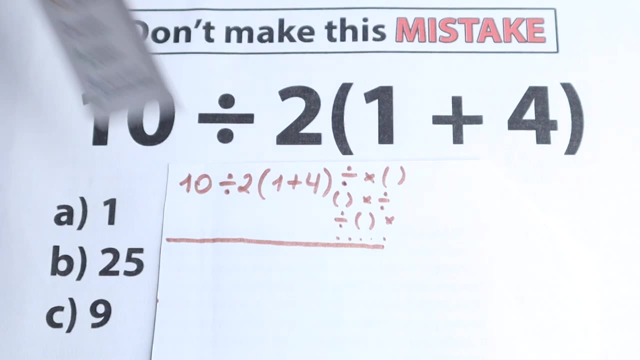 order of operation, because obviously, whatever order of operation we select is going to create a different answer. right In math. we are interested in one correct answer. so let's look at this order of operation I have for this question. I have this PMDMC order of operation. this is the main, the most popular. 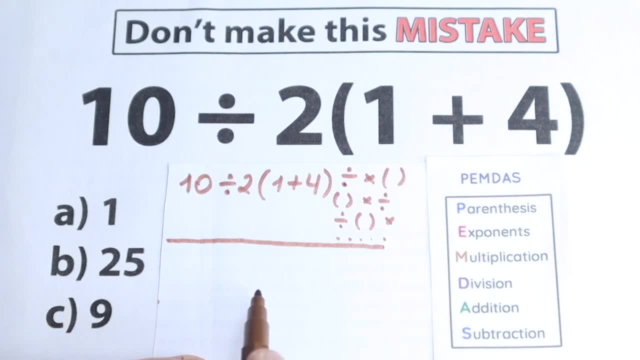 order of operation. in the world, all internet libraries, scientific graphing calculator works according to PMDMC and for this question I prepare this PMDMC paper right here and I want to say that I respect every order of operation. I respect BODMAS, I respect whatever order of operation. 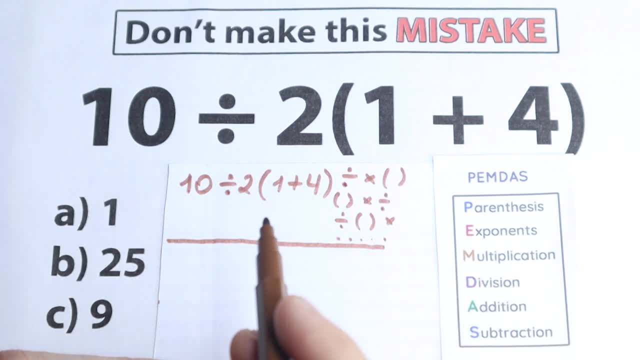 in the world. I respect it because a lot of countries solve it in a different like order of operation, have their own order of operation and I respect it. but I choose PMDMC because this is the most popular order of operation in the world. I learned this. PMDMC and a lot of countries solve. 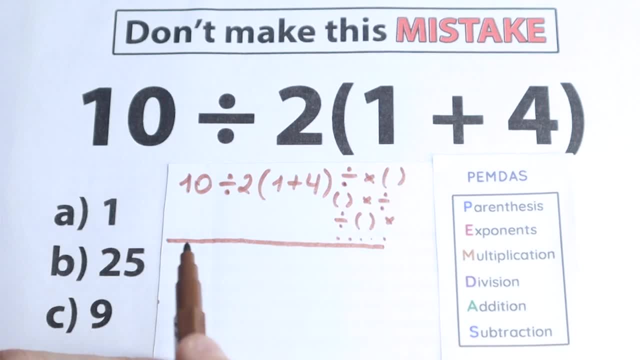 it according to PMDMC, but I respect, for example, BODMAS and a lot of different order of operation, so let's solve it according to PMDMC. So we have 10 divided by 2, and in parentheses we have 1 plus 4.. So, as you can see, right here we 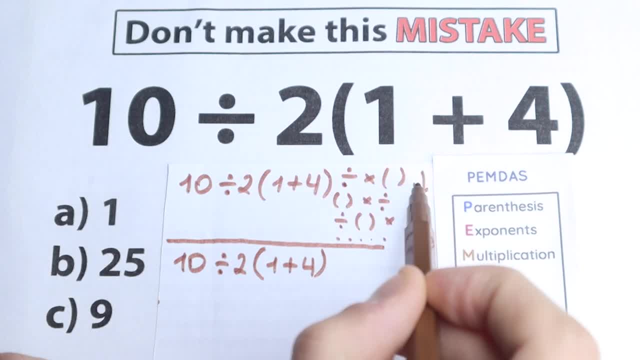 had a lot of combination, but according to PMDMC, we have only one first step. the first step: parentheses. As you can see, right here, we have parentheses. we have this parentheses step. so let's look at it. where do we have these parentheses right here? let's look at it. Yeah, we have parentheses right. 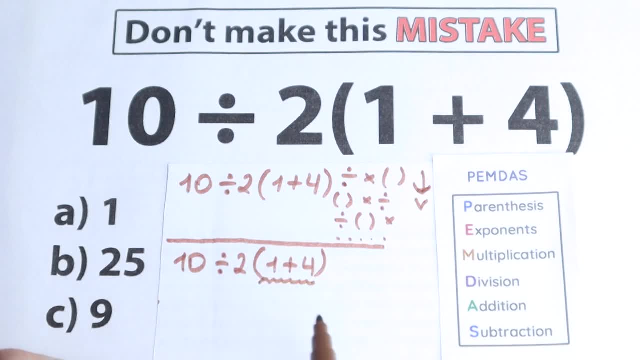 here. so we need to start from it right here. we don't have on the left hand side, we have right here our parentheses. So we have 10 divided by 2 and times 1 plus 4 equal to 5, and this may be the. 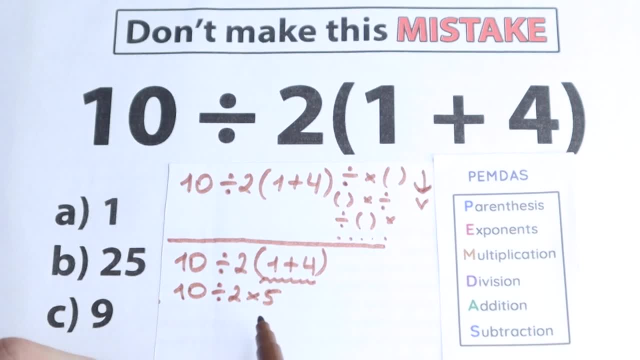 main viral question in the world, because a lot of discussion about it, a lot of discussion about it. So let's solve it according to PMDMC and then division. and I would say I respect every of this order of operation. I respect it, but I will solve it according to PMDMC and I explained to you why. 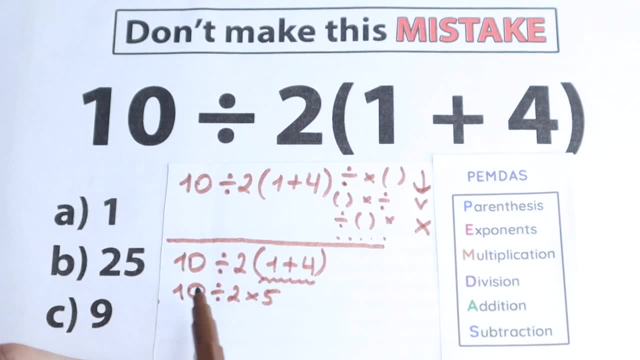 like one minute before. Okay, exponents. we don't have any exponents right here because we don't have any squares. cubes, we have like a regular expression without any powers. Okay, the next step, multiplication. but according to PMDMC, this is a very tricky moment because a lot of students forget. 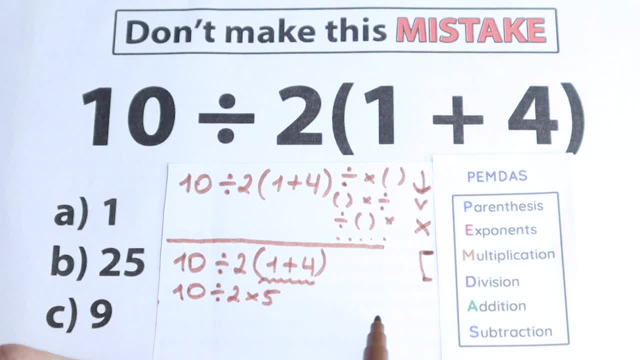 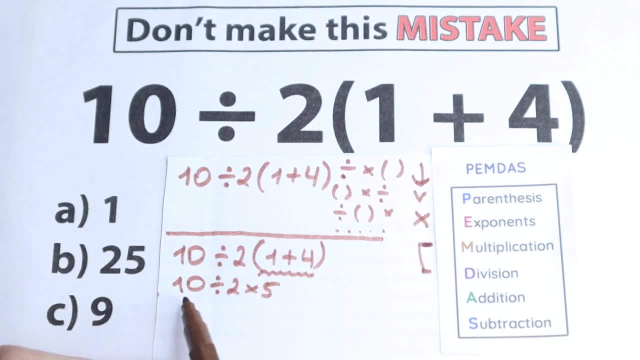 about it. we need to look at it as a group. So multiplication and division- this is like one common thing that we need to scan. where do we have this multiplication and division signs? Let's look at it in the perspective of multiplication and division sign. So right here we have division sign. 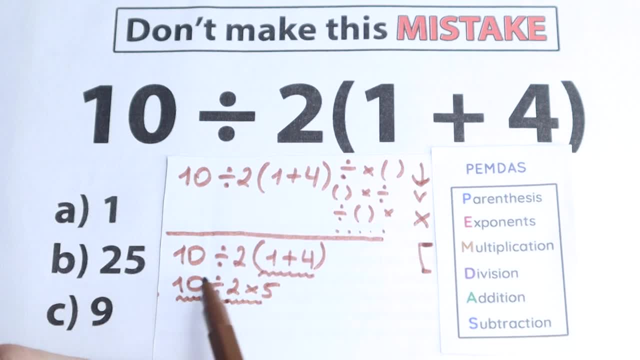 so we need this expression and we still have multiplication sign. So it's really great, all our expression. we just solve it according to this, according to this multiplication and division group. so we have multiplication, we have division group, We don't have addition, we don't have. 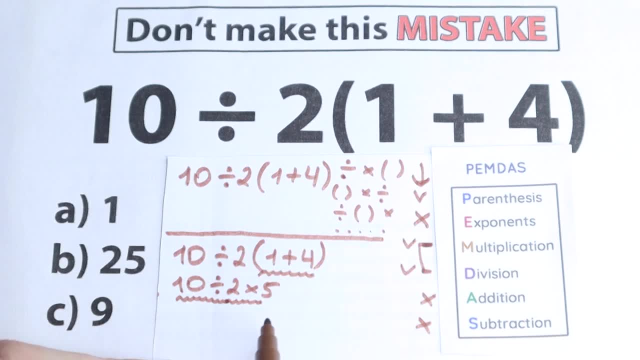 subtraction, so just going a little bit faster. so we don't have it. Yeah, we have only multiplication and division sign. Now I feel one part of you prefer this multiplication at first, because we have, like 10 divided by 2 times 5 equal to 10, so it looks like a is a correct answer for for some countries. I 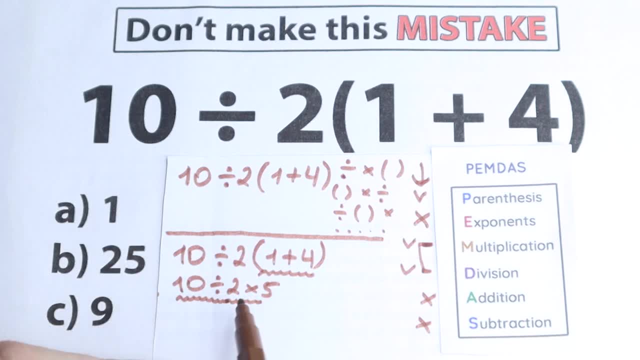 don't know exactly, but some countries solve it according to another order of operation and they say: okay, option a is a correct answer. but according to PMDMC, this is like more easier for us, because we just need to scan what is the first sign. from left, from left to right, We have two signs. this is 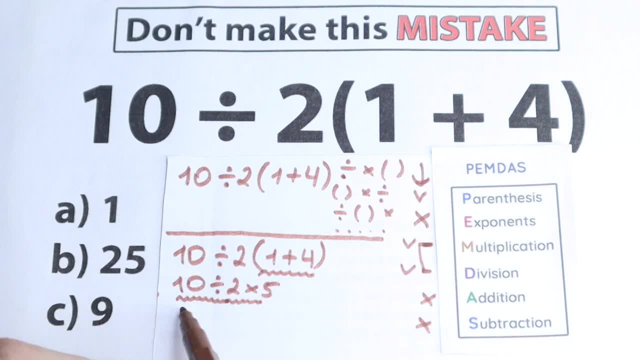 on the right hand side. this is on the left hand side. so right here, from left to right, is the first division, so we need to divide it first. 10 divided by 2. so it is our first step. 10 divided by 2 equal to 5 and 5. with this 5, this is like a basic multiplication equal to equal to 25. this is: 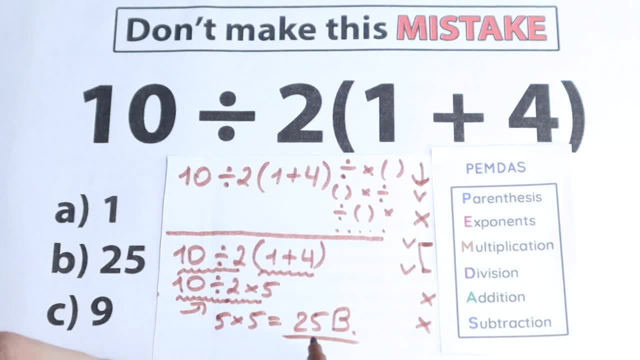 option b. I prefer this option. I solve it like that because I prefer PMDMC. but I respect every order of operation and, for example, if in your country correct answer is option a, I respect it a lot of. a lot of people, a lot of opinions, a lot of thoughts about it. 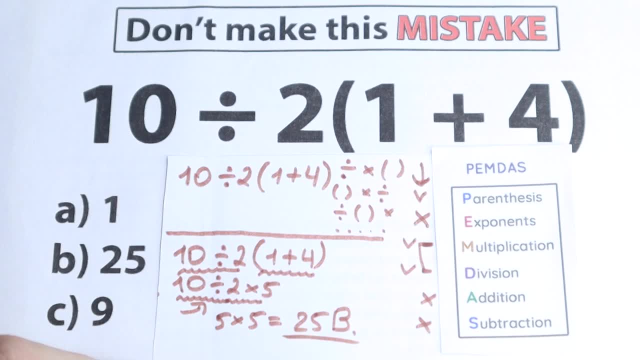 and it's great old people are different, all the countries- maybe some countries are the same, some different, and a lot of countries have their own order of operation and we need to respect it. but I prefer this option, option b. so this is my thoughts about this question. I hope you understand.